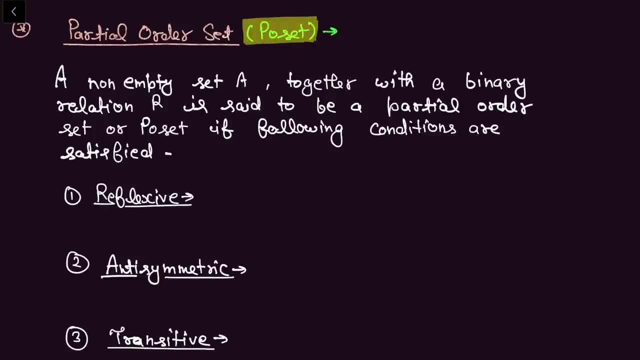 Partial order set is also called poset. in short, When is partial order set made? For partial order set, we will take a known empty set, capital A. For partial order set, we will take a known empty set, capital A, Together with binary relation. We will take a binary relation and name it capital R. 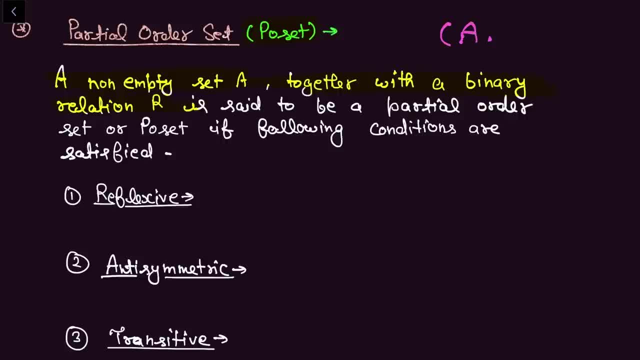 If we write A set with its relation, Then it becomes partial order set. We also call it poset. If it satisfies some conditions, Is set to be partial order set or poset If following conditions are satisfied: If following conditions are satisfied, Then we will call this pair of A and R as poset. 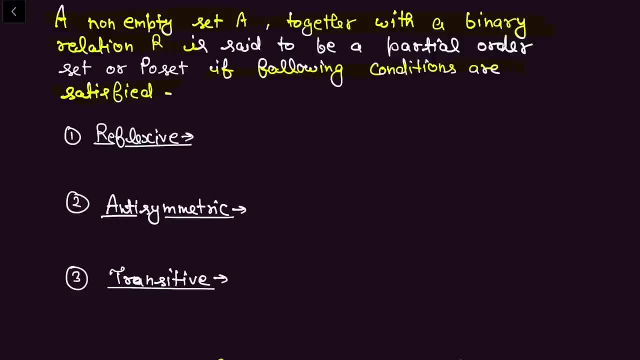 Right. So poset depends on relation. So relation satisfies three properties. First property is reflexive. Second is anti-symmetric. Third is transitive. So relation R is defined on A set. If it is reflexive, anti-symmetric and transitive, Then it becomes partial order set. 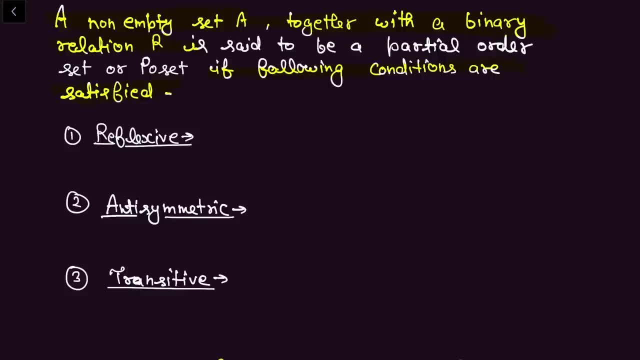 And if we write A set as a pair with R, Then it becomes partial order set, Right? So if we want to show R as reflexive, Then we will use the same condition of first module, Right. In first module you learned that The pair of A and A is related to our relation. 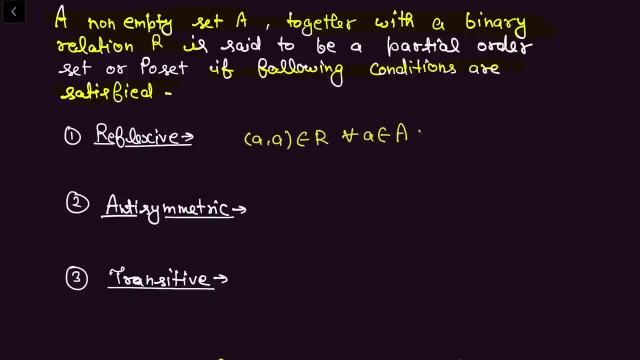 And this condition is: for all A belongs to A. Or you can write it like this, That A should be related to A only For all A belongs to A. Both have the same meaning. So if this condition is satisfied in our relation, Then that relation will be reflexive. 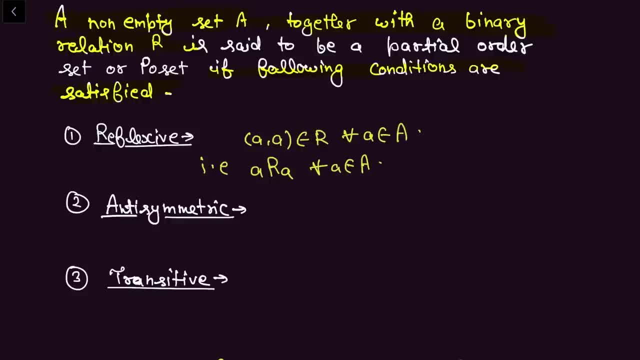 Then let's talk about anti-symmetric. Right? What happens in anti-symmetric? In anti-symmetric, if we have two elements- One element is A And one element is B, And both belong to our set A- Then At the same time We say that: 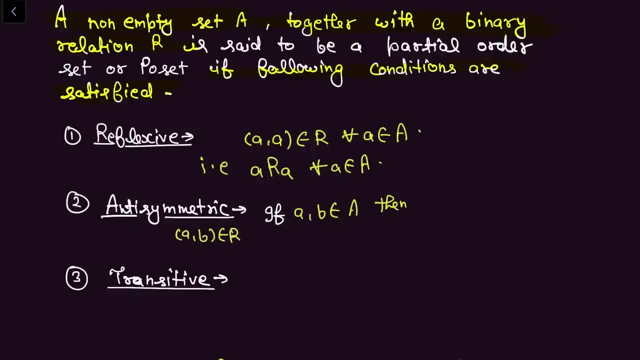 A and B belongs to R And at the same time B and C. Sorry, B and A belongs to R Means R belongs to our relation. Relation is the set of an order pair. As you know, Right, A and B belongs to R And at the same time, B and A belongs to R. 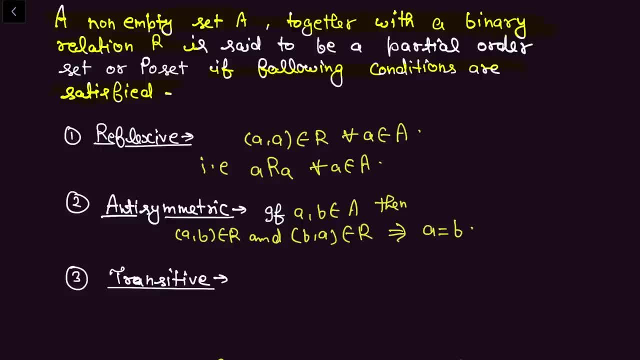 So this implies that The element A should be equal to B. This property is called anti-symmetric property, Or we can say it like this: A is related to B And B is related to A, So this possibility is created When A is equal to B. 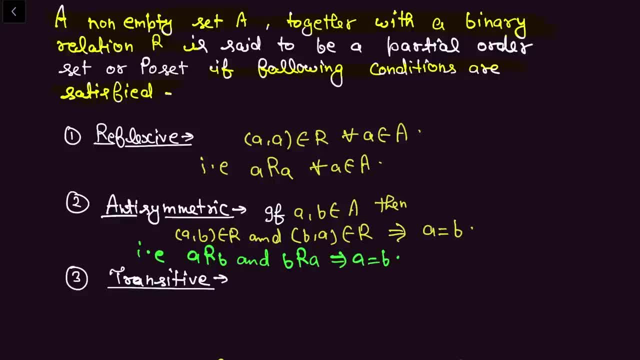 Right, So this property is anti-symmetric property. Then the third property is transitive. In transitive we take three elements. We take A, B and C And all three elements belong to set A. All three elements belong to set A And the property of transitive says that. 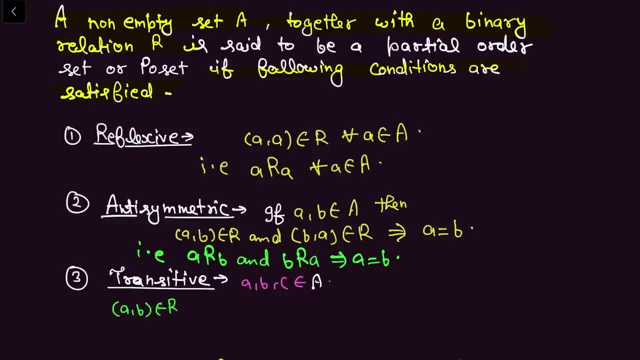 If A and B belongs to our relation, R And B belongs to R, by making a pair with C, Then the middle element B is eliminated. The pair of A and C will be made. So the pair of A and C will be made. This is the middle element. 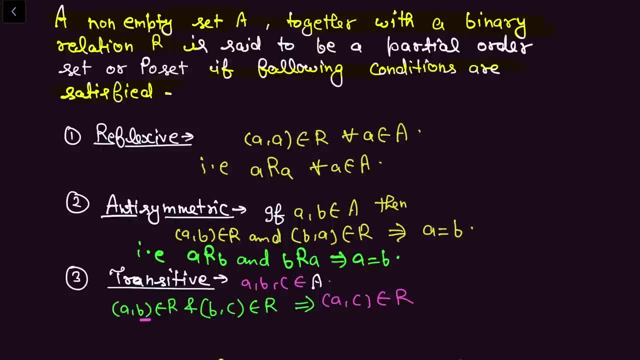 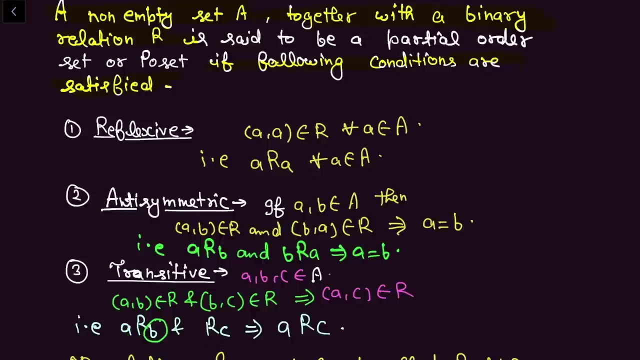 1 And 1 Will be made, and this is the middle element. 1 Is the middle element. 2 Will be less than 2, 3 Will be equal to 2, 4 Will be equal to 4. If we make pair with A, A becomes related to C, then we say that our R relation is transitive. 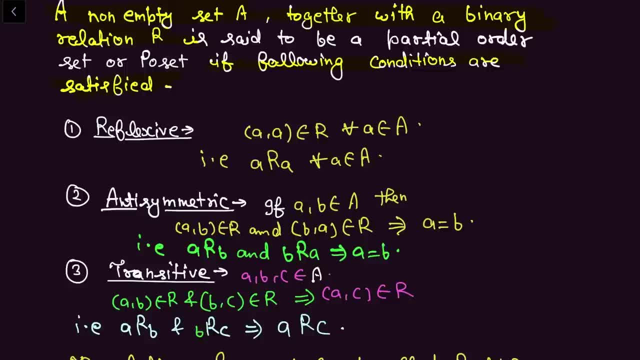 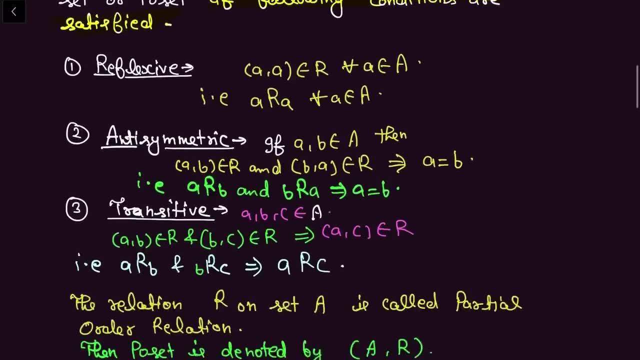 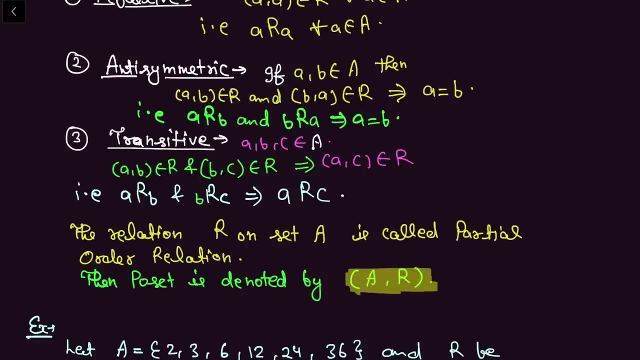 if we satisfy this property. So if the R relation satisfies these three conditions- reflexive, anti-symmetric and transitive- then it is called our partial order relation. and if we make a set with this R relation in this way, if we make a set with this R relation in this way, if we make a 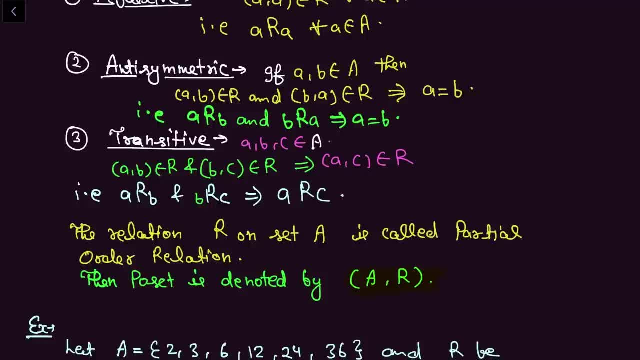 set with this R relation. in this way then it is called our partial order set. We are going to define the lattice with the definition of partial order set. So it is important to know the poset. So always keep in mind the poset. 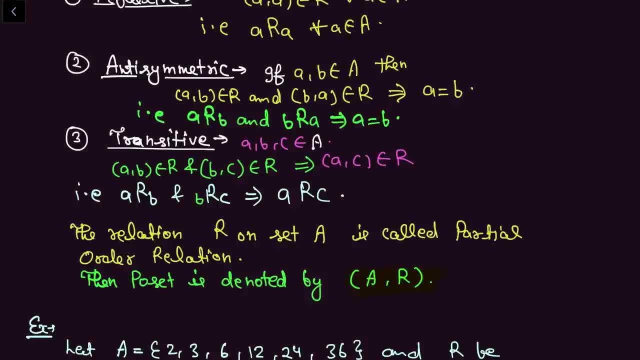 If we make a set with a relation in this way, what is the relation? If the partial order relation is there, that means it holds the reflexive anti-symmetric transitive property, then we call this pair poset or partial order set. 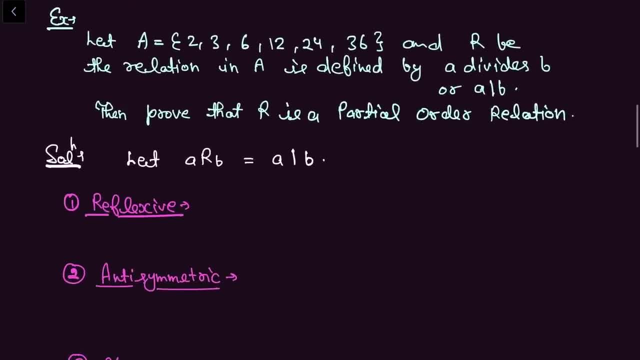 Let's take an example. We have taken a set A, capital A, which has elements 2,, 3,, 6,, 12,, 24 and 36.. This is our set A And our R relation is on this set, on A set. 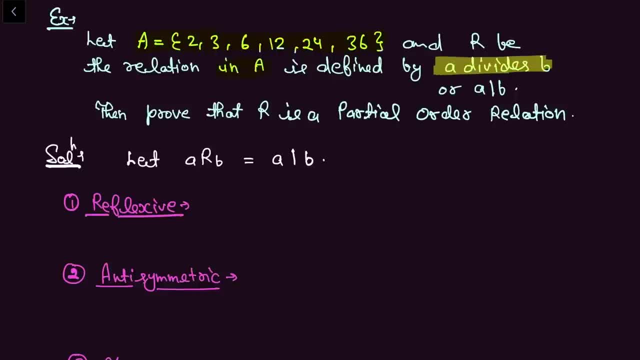 And how is it defined: A divides B. This is how it is defined: A divides B. A divides B means B divides A. We can write this in three ways. One way is this, Or we can write it like this: A divides B. 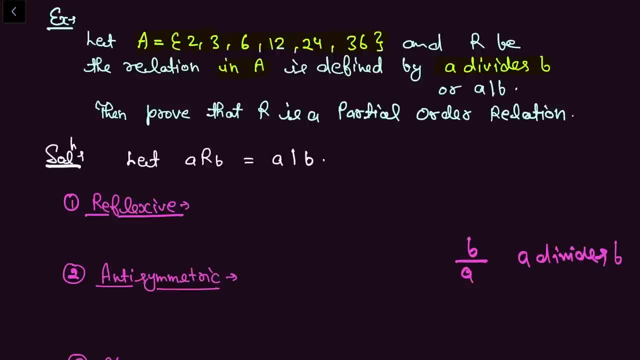 Or we can write it like this: B upon A. Or we can write it like this: This is the standard way: A divides B. We will write A. We will put a straight line B. This means that A divides B. 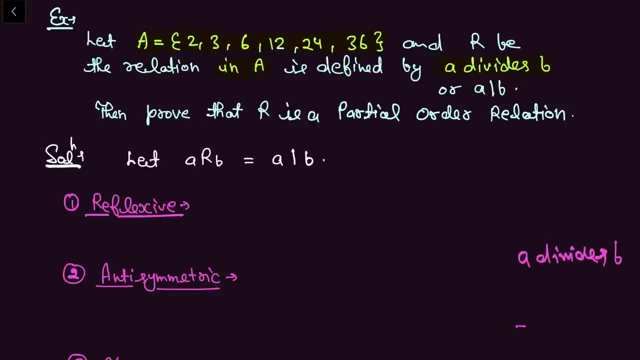 We call this: A divides B, Which simply means B upon A. So the relation here is the relation of divide. The relation of divide is on this set. Then we have to prove that if we take the relation of divide Then this R relation will make a partial order relation. 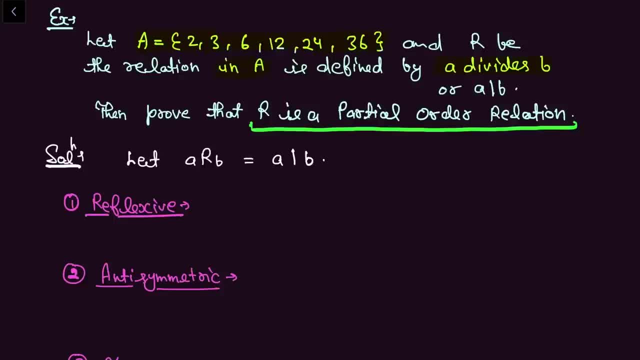 And along with this, this A set will make a partial order set with R. So first we have defined that, the relation R here. If we say A related B, It means that A divides B, A divides B. Okay, What will be the meaning of A related B here? 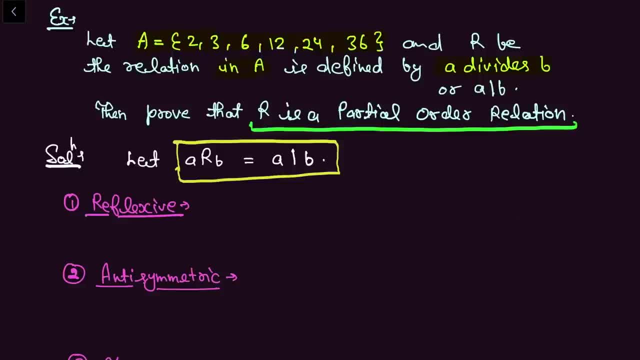 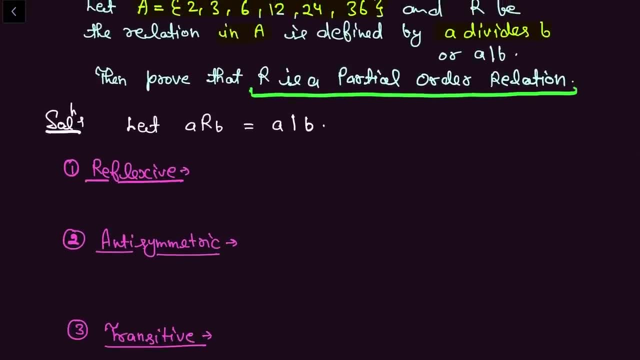 A divides B. It means that A divides B. We have understood this. Now we will prove this relation as Reflexive, Symmetric and Transitive. Okay, We will prove these three properties in this. The relation of divide. You all know that any element always divides itself. 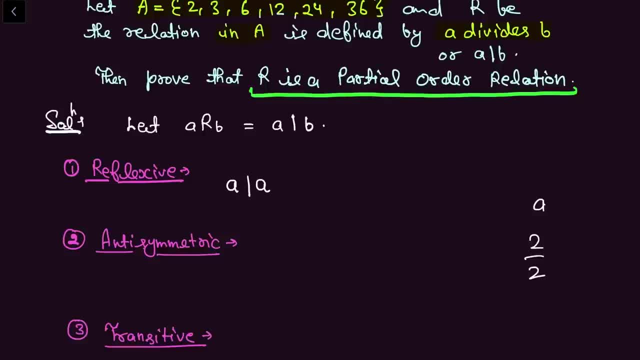 A will always divide itself, Like 2 divides 2 and gives 1.. 3 divides 3 and gives 1.. Isn't it? So any element always divides itself, Isn't it? If A divides A, Then you can say that here A is related to A. 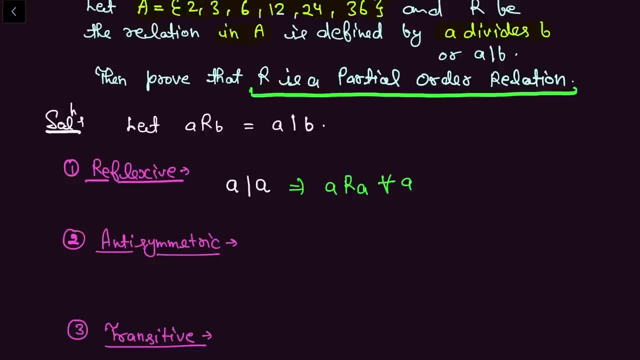 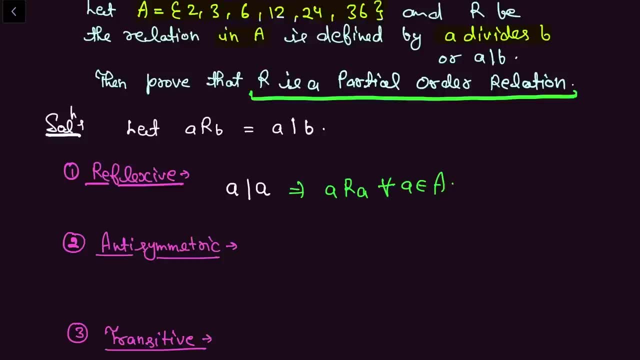 And this condition can be done with any element, Isn't it? The element in A set is 23,, 6,, 12,, 24,, 36.. The condition will be satisfied for all, Isn't it? And what is this condition? 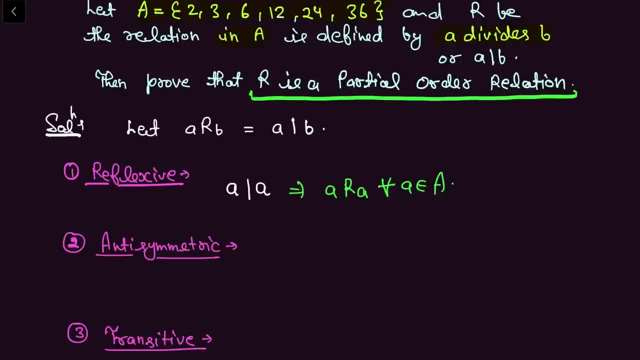 This condition is Reflexive property. Okay, We can write it by doing, since, Because we know that any element always divides itself, it means that A will relate with A and this R relation will be reflexive. in this case, R is reflexive. 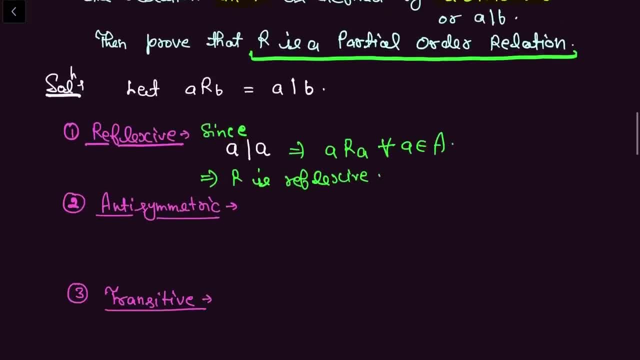 This is the property of reflexive. Second is anti-symmetric property. You always know the relation of divide in the relation of divide. If you say that A divides B and you also say that B divides A, then when is this possible? This is only possible when A is equal to B. 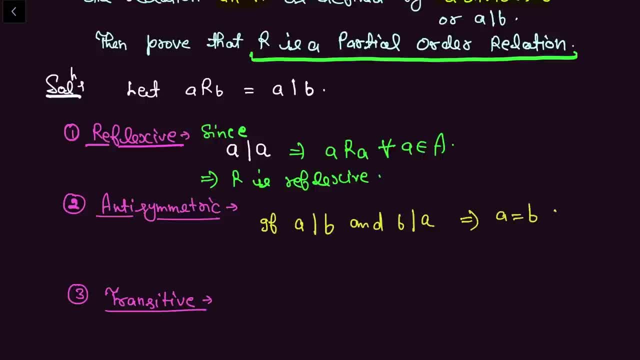 This is only possible when A is equal to B. You can say that if A relates with B and B relates with A, then this is only possible when A is equal to B. And what is this condition? This condition is anti-symmetric. 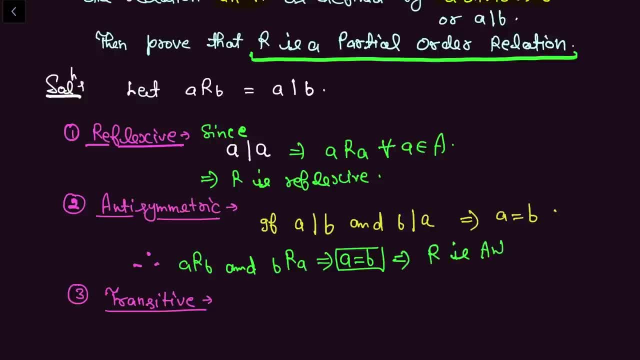 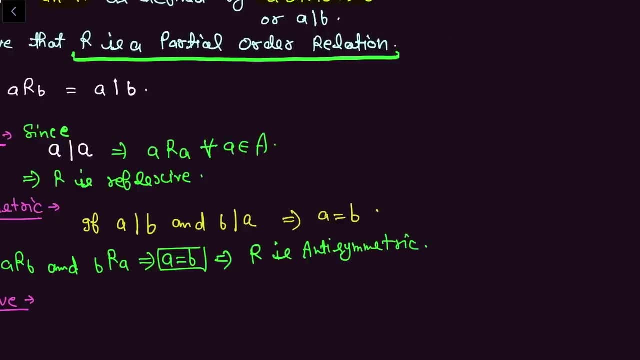 You can say that R is anti-symmetric. You can understand this by example. You can take any particular example. For example, you said that 2 divides 3.. Then you say that 3 is. Sorry, I wrote it upside down. 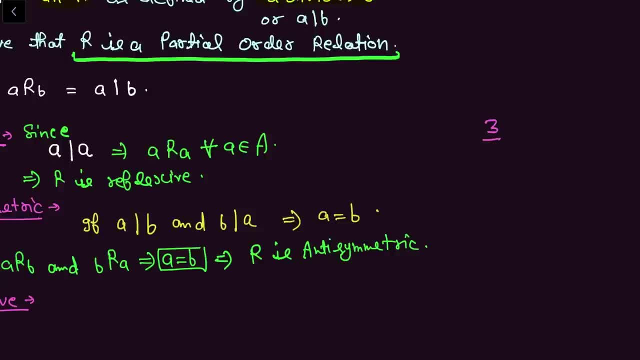 You said that 2 divides 3. This means 3 by 2.. You said that 3 divides 2.. So what can be equal in this case? 2 will never be equal to 3.. But there is one possibility. 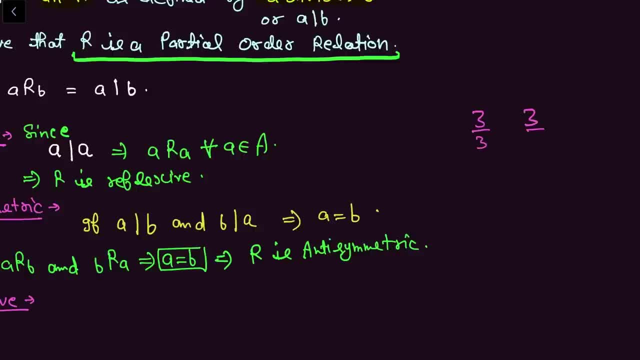 If we say that 3 divides 3 and 3 divides 3, then this is only possible if the values of A and B are the same. We have written that in the relation of divide. if A divides B and B divides A. 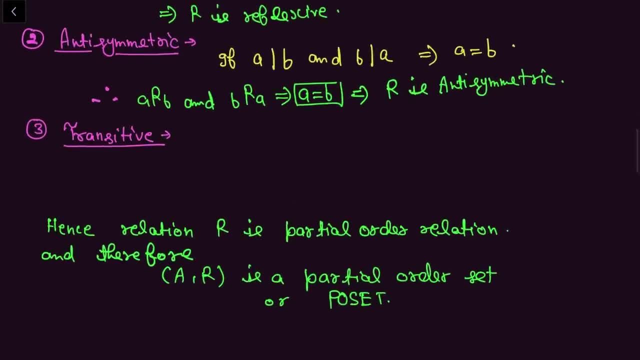 then this possibility can only come when both the elements are equal. Otherwise the possibility never comes. So in this case our relation will be anti-symmetric. Let's talk about transitive property. You know transitive property very well in divide. 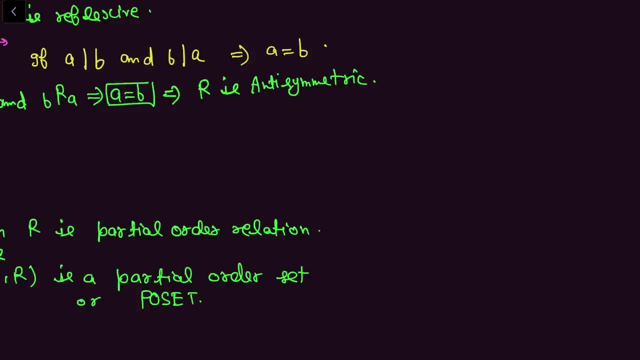 If you say that there are 2 elements in the set, There are 3 elements, 6 elements, 12 elements, 24 and 36.. Transitive property: If 2 divides 6 and 6 divides 12, then definitely this 2 will also divide this 12.. 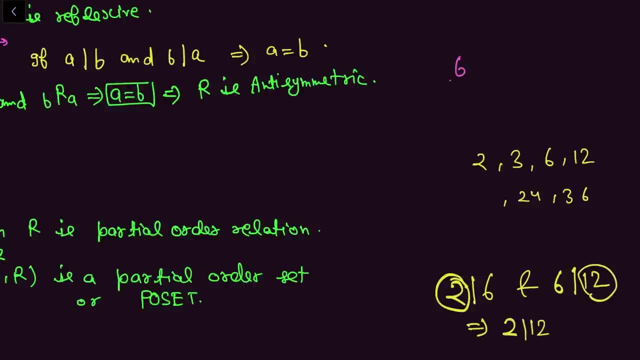 And this is your well-known result. If you divide 6 by 2 and 12 by 6, then definitely this 2 will also divide 12. It does So. in this divide, your transitive property will be easily held for the set. 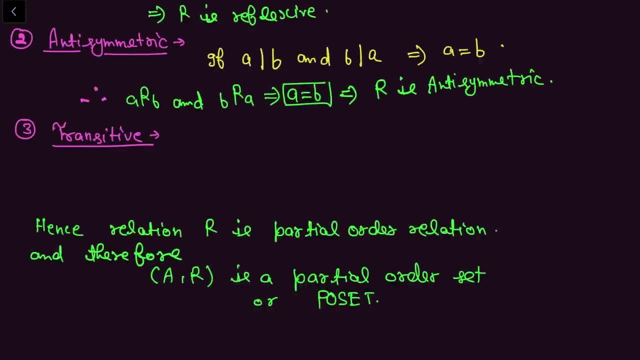 So this is what you have to write in transitive property. We have assumed that A, B, C are 3 elements. A, B, C are 3 elements that belong to A set, And we have considered that A divides B and B divides C. 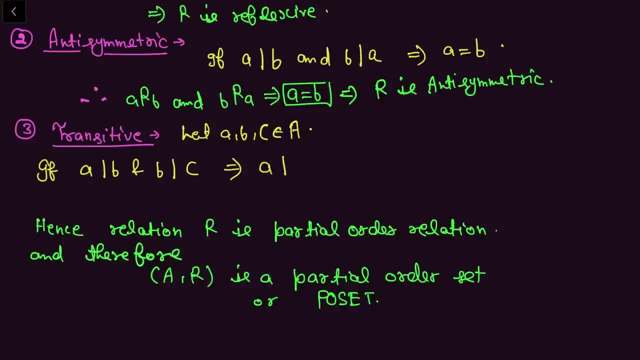 If so, this implies it will definitely happen in the relation of divide that A will also divide C. Okay, That means you can say that if A relates to B and B relates to C, then this middle element will be hide and A will relate to C. 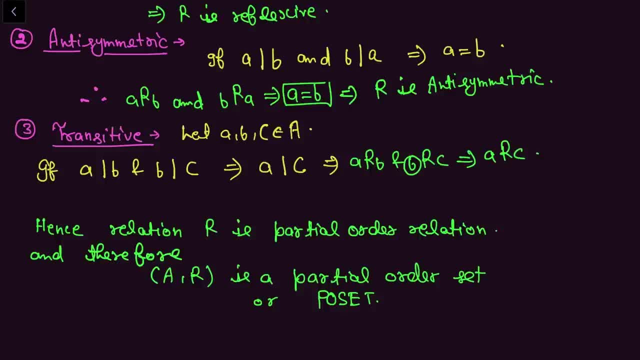 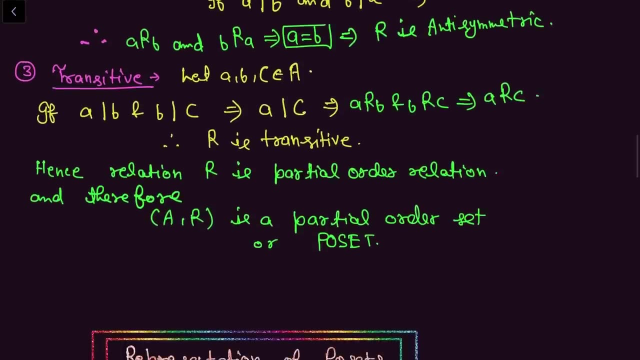 This means this will happen And this is our transitive property Right. Therefore, you can write that R is transitive, R holds the transitive property. Okay, That means this relation, this divided one, this will be our partial order relation. 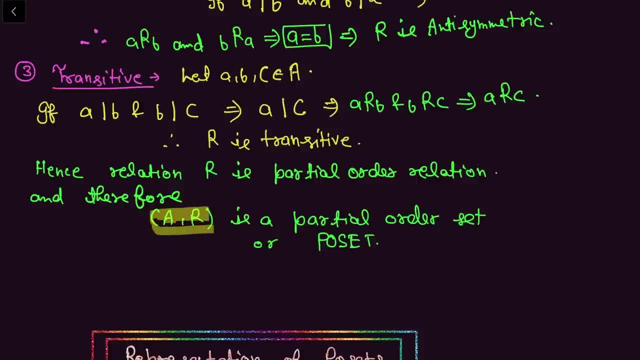 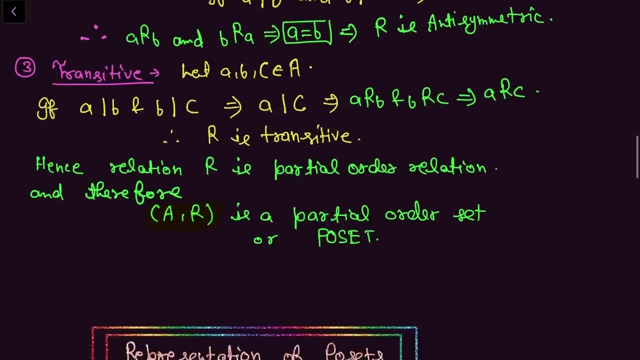 All three properties have been satisfied And the pair of A will be made with this relation. that is our partial order set, which we will call poset. So this example will be of our poset. So this is our poset. When does our poset become our partial order set? 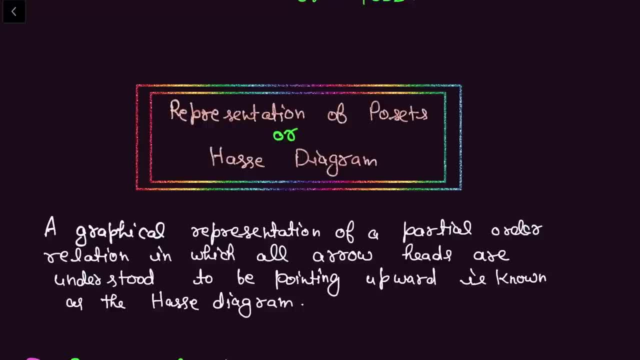 Now we can represent this poset graphically, Right. We can also make a diagram of it, Right, Because things become very easy with a diagram, Right? You can do very big calculations with a diagram very easily. So we will learn to represent the poset by a diagram. 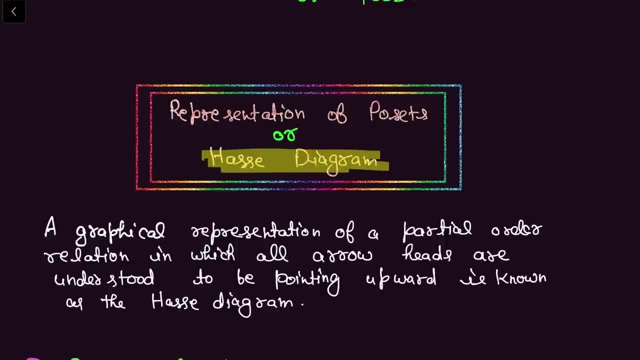 And this diagram we call it as a hash diagram. Okay, Which diagram will we call it Hash diagram? You are given a hash diagram in lattice And you have to check whether it is our lattice or not. So first you should know about the hash diagram. 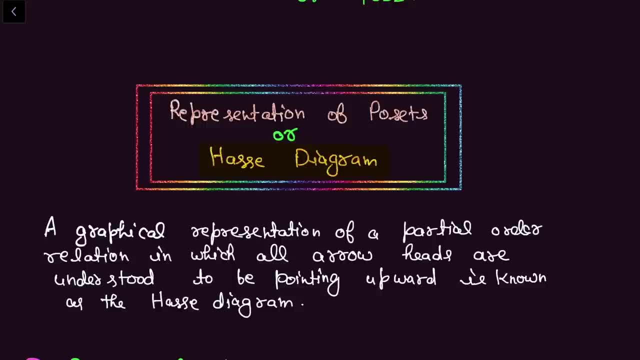 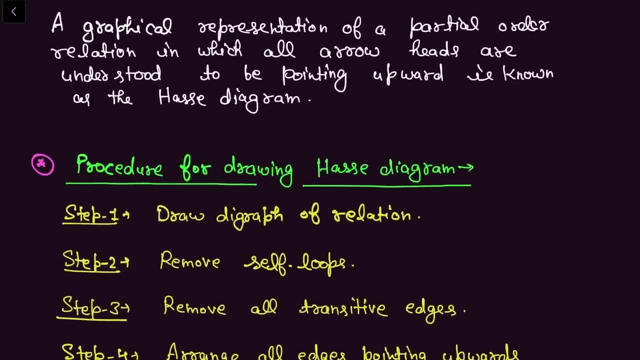 Because sometimes you have to make a hash diagram to prove the lattice. That is why it is important to know about the hash diagram, Hash diagram. I have simply told you that if we represent the poset graphically- a graphical representation of a partial order relation- 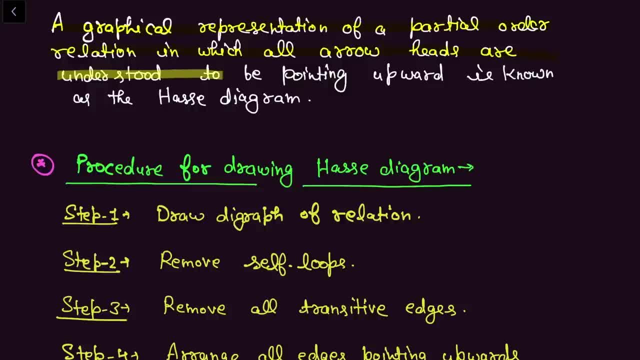 in which all arrows heads are under to be pointing upwards, is known as the hash diagram. So we represent the partial order relation or partial order set graphically Right In which the arrow heads- because first we make a diagram in it. 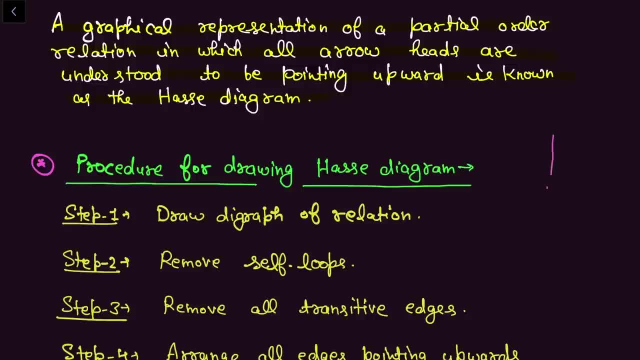 Right. We make a diagram And in the diagram if A is related to B, then we show it in this way with an arrow, So the arrow heads. we always try to keep it upwards Right. So the diagram that is made in this way. 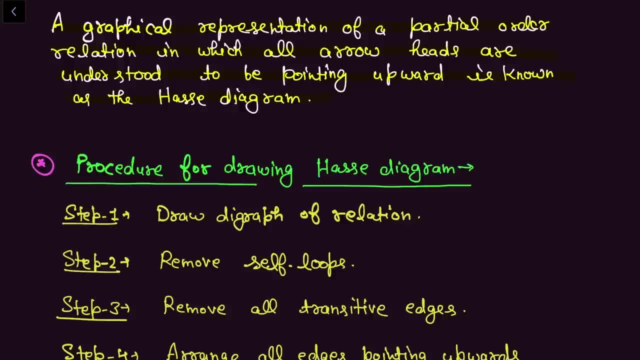 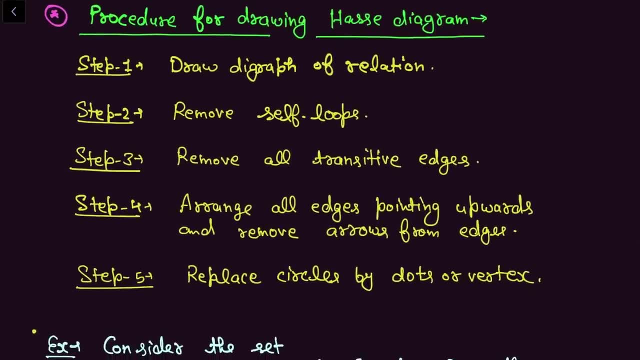 will be our hash diagram. You will understand better than the example. There is a process of making a hash diagram. Right Processor for drawing hash diagram. Basically it is done in four steps. The main step is only three steps. The other two steps are for formality. 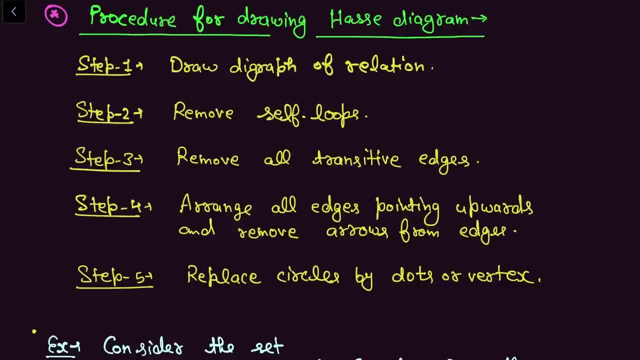 For the last Right. So our first step is that we have to make a diagraph- Directed graph, which is called draw diagraph of the relation Right, We have to make a diagraph or a directed graph, Directed graph which I had taught you to make in module 1.. 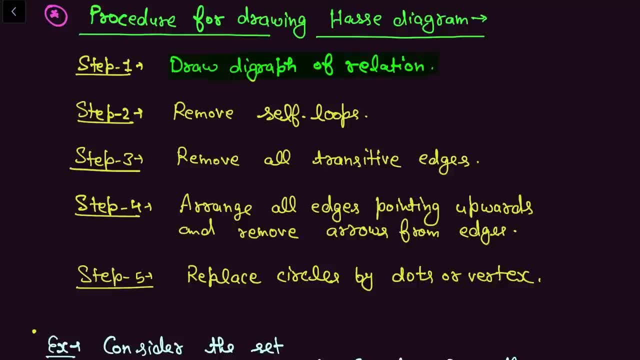 We have a relation, Its elements. we write the elements of the set in a circle And then the ones that relate. we define them with an arrow, So that becomes a diagraph. So first of all I have to make a diagraph of the relation. 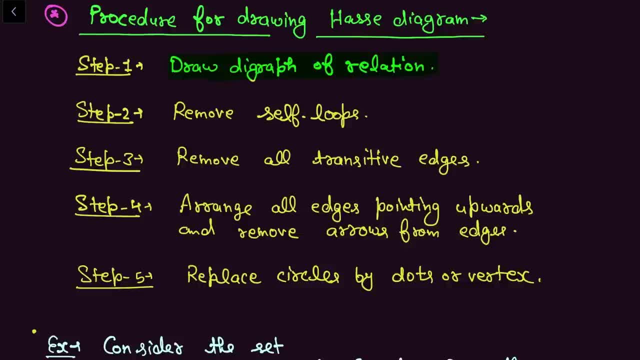 If you do not know how to make a diagraph, then I have made a particular video of it in module 1.. You can learn it there. Then in the diagraph, our parallel ages self loops all come, So we have to remove this self loop. 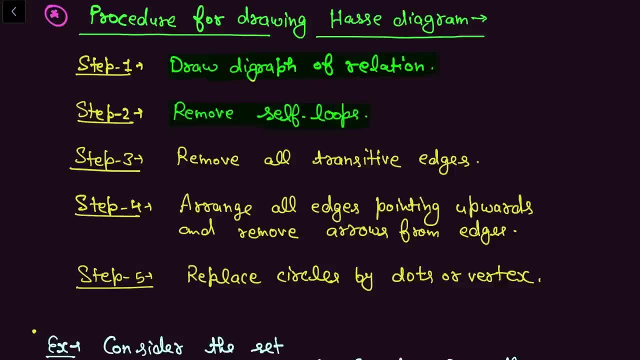 in the second step, All the self loops will be. Self loop means a cycle of this kind. For example, there is an element A. After moving from the element A, yours ends on it. So this is called a self loop. We have to remove them. 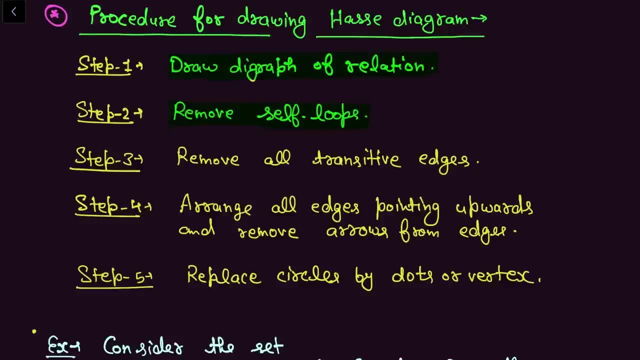 We have to delete them from the diagram. This will be the second step. In the third step, all the transitive ages will be After removing the self loop. we have to remove them. Okay, Self loop means the reflexive property that is held. 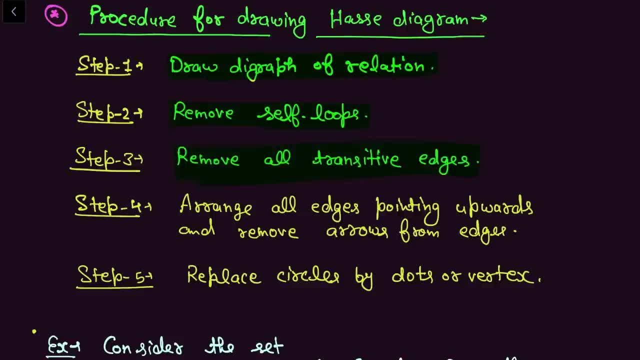 that makes the self loop Right. So after removing the self loop, the figure that will be made, all the elements that will be left in the set. we have to see in them which elements hold the transitive property, So the transitive ages that will be made from them. 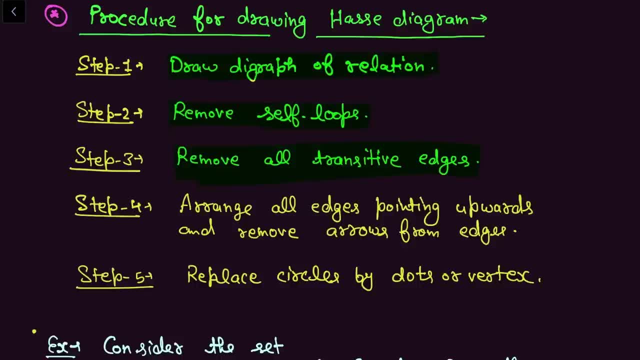 we have to remove those transitive ages. We have to eliminate them from our graph. And in the third and fourth step, what we have to do is the arrows. we have to remove them and make them an age. We have to make a straight line. 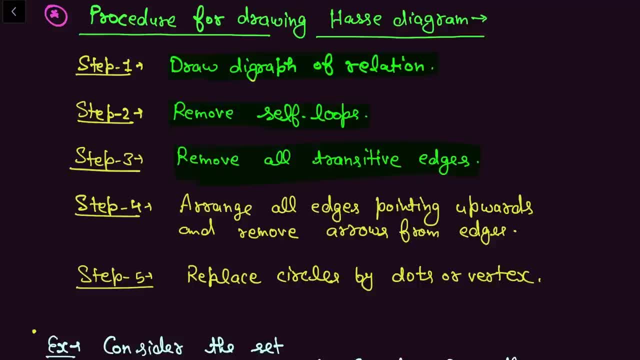 And the circles that will be there, in which the elements will be written. we will represent them with a dot Right And we have to try that the notation of the arrows will be upward. We have to point them upwards Right And according to that, 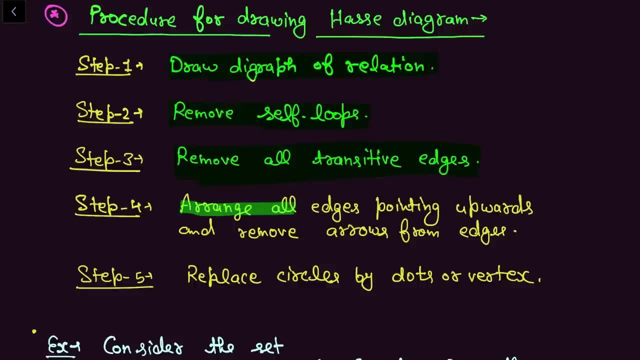 we have to put an age later. So in the last step we remove the arrows and make them ages, And we have to make the circles with dot or vertex, And in this way our Heisei diagram is made. Let's take an example. 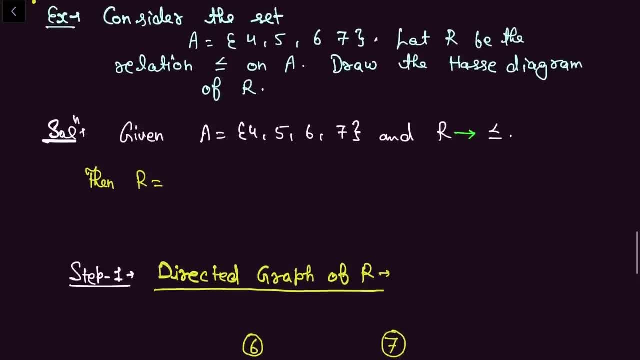 I will tell you all the steps clearly. I have considered that I have A set In A set. our element is 4,, 5,, 6,, 7.. And R is our relation. The relation is less than or equal to. 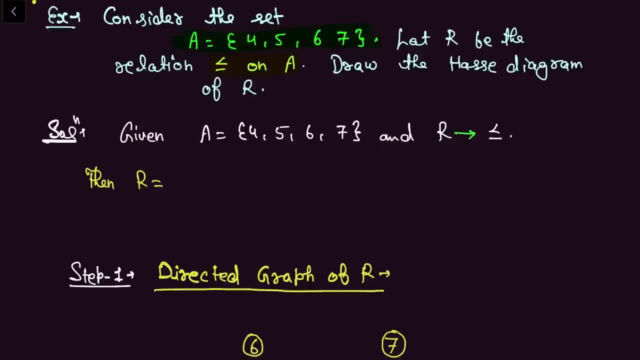 In this set the relation is defined between elements less than or equal to. So we have to make a Heisei diagram for this relation. Right? This is a poset. A poset will always be made here. You can also prove it as a poset. 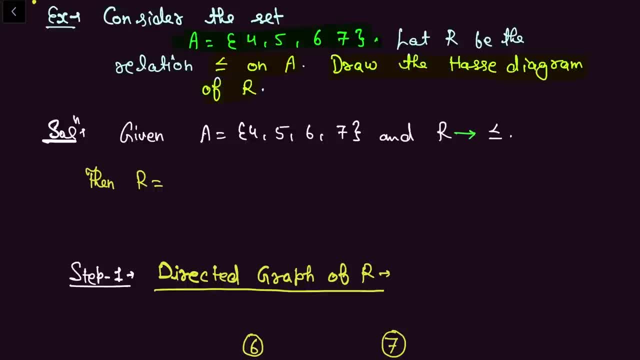 Then for this we will make a Heisei diagram here. First of all, to make a Heisei diagram we need relation R, That is, which elements will belong to relation R? Our relation is represented here by less than or equal to. 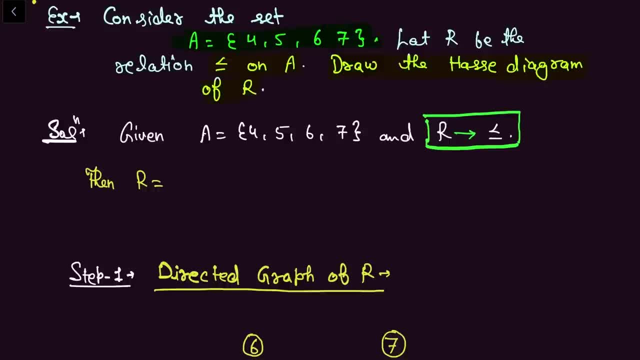 So in the elements you have to see the condition of less than or equal to. Which elements are there? They will relate to each other. Let's make a set of relation R. What will be made? Let's see the self elements first. 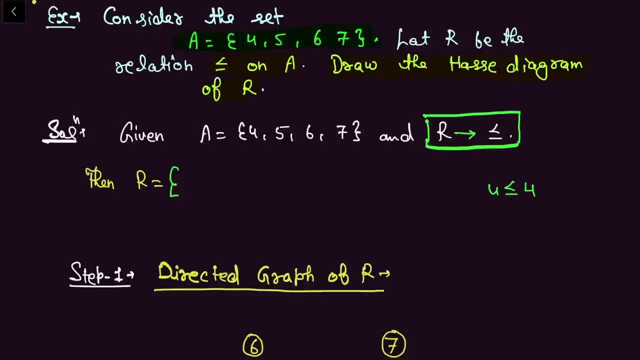 Is 4 less than or equal to 4 or not? Yes, it is, because it also has an equal sign, So 4 equals 4.. That is the 4. 4 element will belong to our relation Right? Similarly. 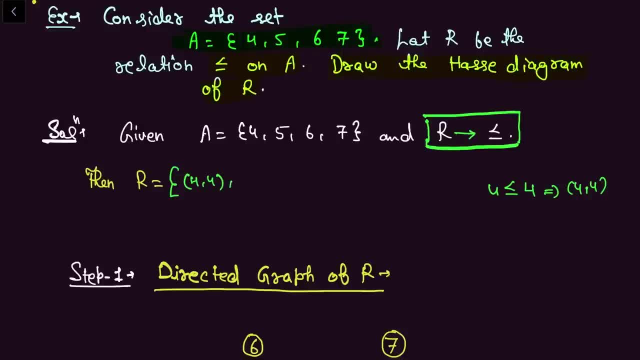 if 5 is less than or equal to 5, then 5- 5 element will also belong to our relation. If 6 is less than or equal to 6, then 6- 6 will also belong to it. That is. 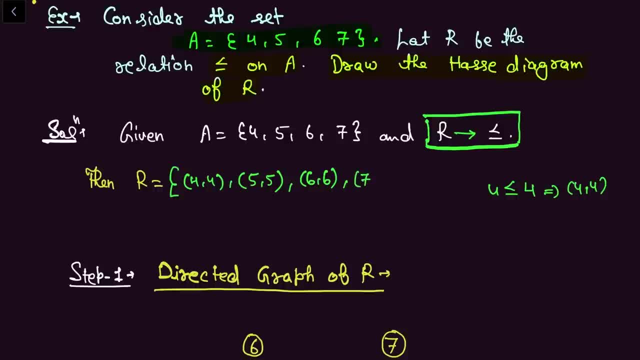 we will relate to each other in this way And 7- 7 will also be our relation. in this relation, Because it is a poset, the reflexive property will always hold. With the reflexive property, these four elements will be made here. 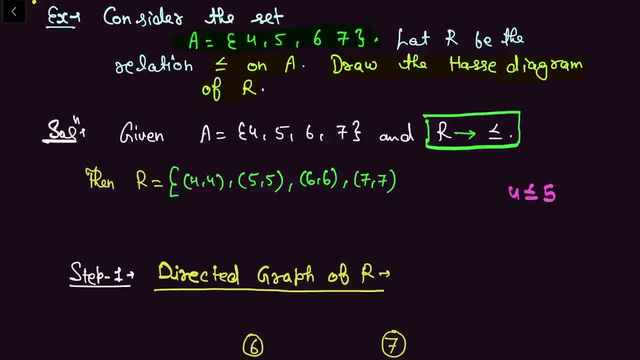 Now we have to see one element: If we talk about 4, then 4 is less than or equal to 5.. Yes, that is 4. 5 will belong to our set. Then 4- 6 also satisfies our condition. 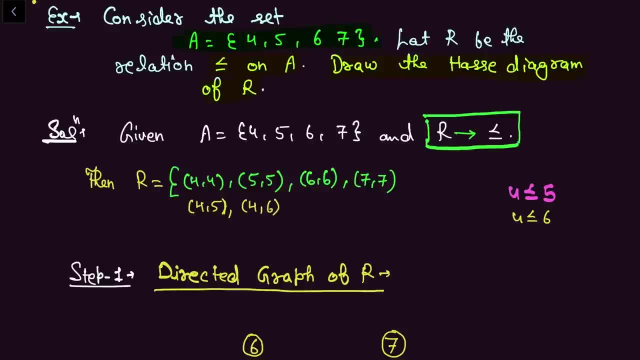 So it will be related to 4- 6. That is, 4: 7 belongs to this condition, Then 4: 7 belongs to our relation too. Likewise, 5- 6 also satisfies conditions. 5 is less than and equal to 6.. 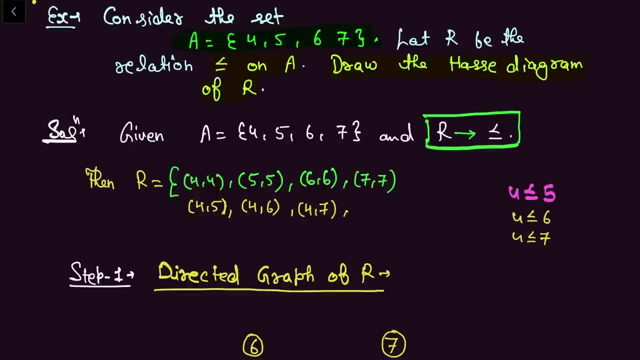 Then it will belong to 5- 6.. Likewise, 5- 7 belongs to our relation as well. And then we talk about 6 and 7. in this relation, 6 is less than or equal to 7. That always happens. 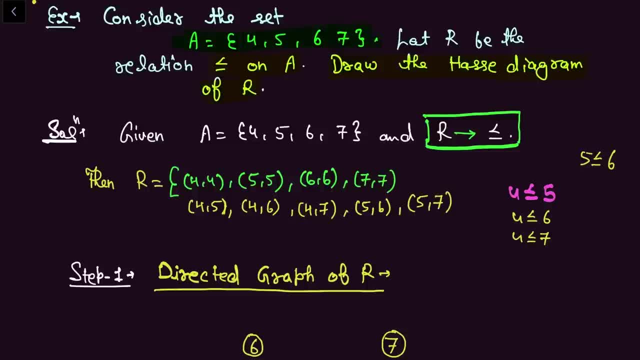 Then it will be related to 6- 7. And 6- 7 belongs to our relation, So we can also see why it is not related to 5- 7.. Let's talk about 6. We will see 6- 3. 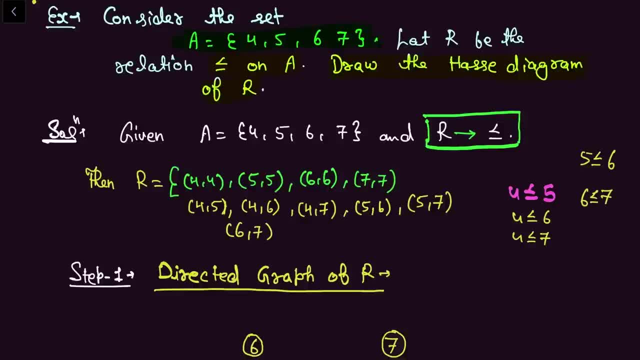 4 equal to 1 will also belong to the set here. okay, so you have to see that in less than equal to elements where this condition can be satisfied, wherever this condition will be satisfied, our relation R will be made. in relation R, our total elements will be made, which I have written here. now we have 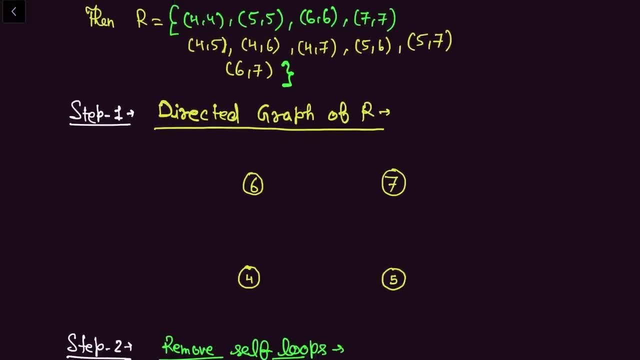 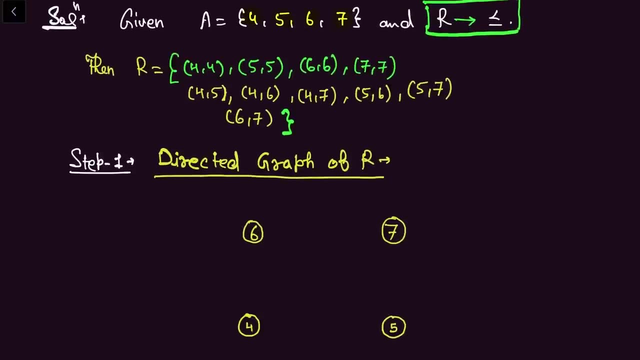 to make the directed graph of this relation. first, to make the directed graph, we will see the elements of the set A. set A has elements 4, 5, 6, 7, write those elements in the circle in this way, as I have written. 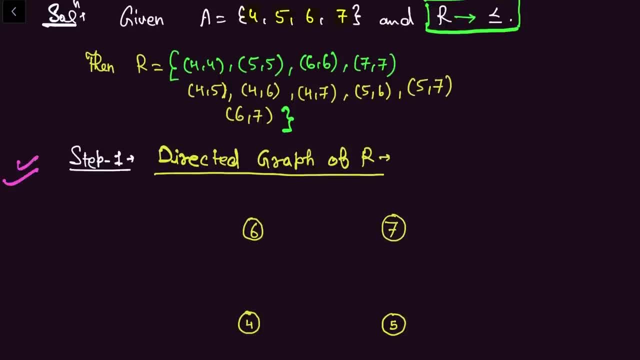 4,, 5,, 6, 7, in step 1,. okay, the method of making a directed graph which I told you in module 1, first write 4,, 5,, 6,, 7 in the circle which is the element of A. now you have the relation. 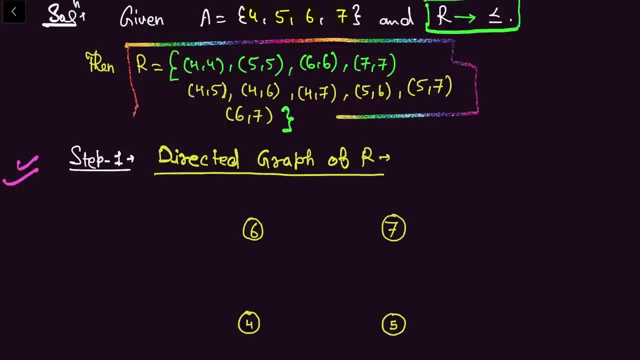 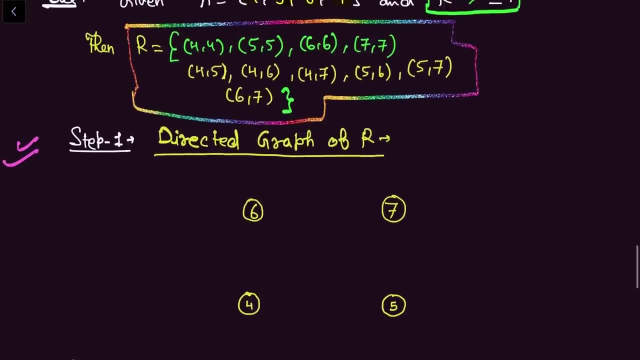 R. its set is made above. looking at that set, you have to put an arrow here. how will you put the arrow? 4, 4 belongs to our set, ie 4 is relating with 4, then a self-loop will be made here and that self-loop will be made in this way. 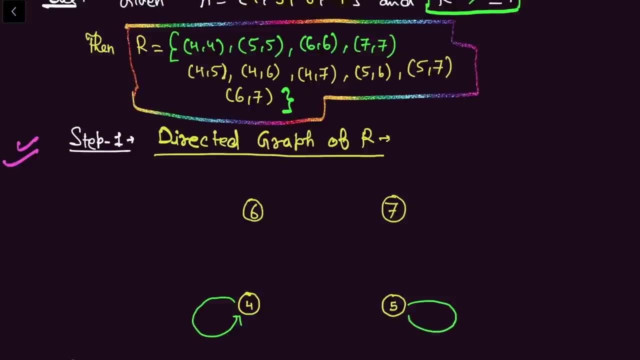 similarly, number 5 also belongs, then a self loop will be made on it also. similarly, number 6 and 6 will also belong in. like this, R will become a such 7 self-loop For all four elements: 3,, 4,, 5, 6, l. 7 will become a single self-loop. If you make a morning 14, after this you will get. Please subscribe to our channel. see you again next time. for all four elements. there should also be a self-loop of R, a self-loop of R, a self-loop of R, a self-loop of At, and for a self-loop of R, a self-loop of 4, five G is. 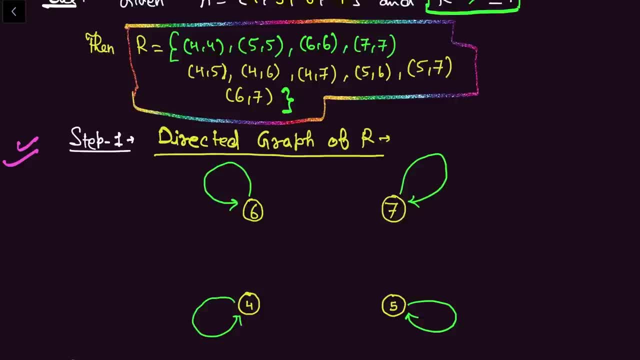 For 4, 5,, 5, 6, 6,, 7, 7, we will make a self loop. we will put an arrow in this way, then the next element is 4,, which is related to 5, so if 4 is related to 5, then we will put an arrow in the middle of 4, 5 in this way and put a line. then 4, 6 belongs to our set in relation r, then 4, 6 will also put a line in the middle of 4, 6,. 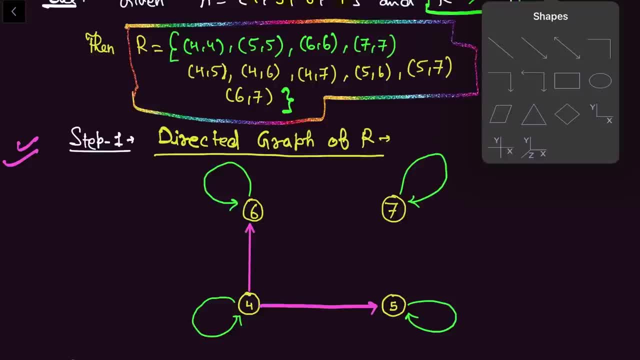 this way, arrow while putting. then 4, 7 also belongs to our set, so we will put a line in the middle of 4, 7 in this way. 4, 7 after 5, 6 belongs to our set, so we will put a line for 5, 6,. 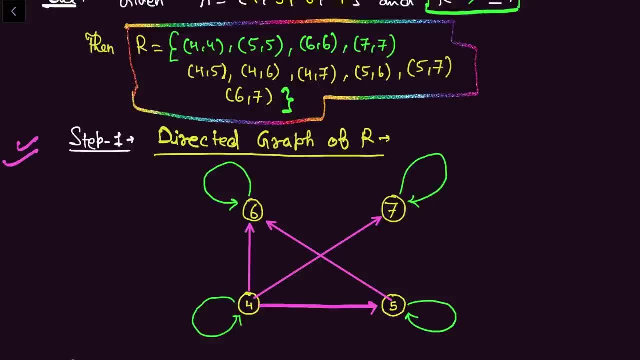 5, 7 belongs to our set. we will put a line for 5, 7 in this way while put an arrow. the last element is 6, 7 belongs to our set, so, starting from 6,, we will put a line on 7 in this way. 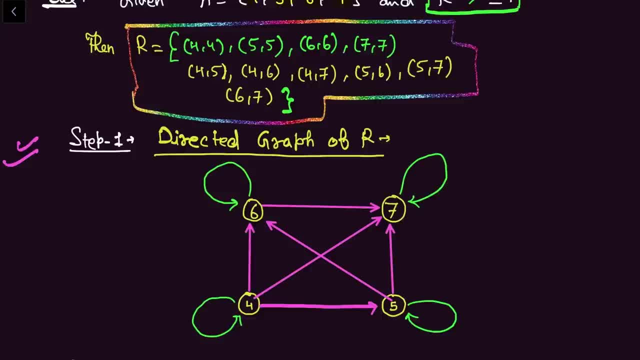 so this graph that we have made it works as directed graph or digraph for this relation. I have taught you how to make this in module 1. so what we have to do in step 1, whatever relation we will make- we have to make a digraph or directed graph like this: 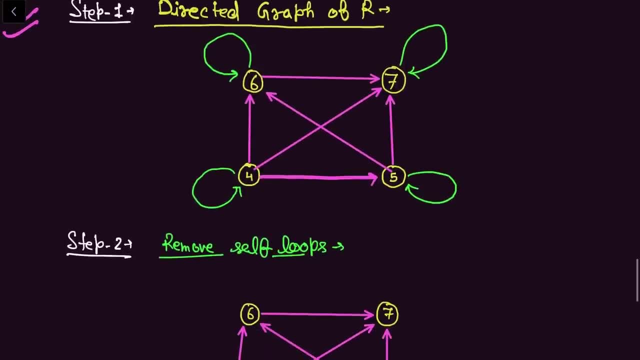 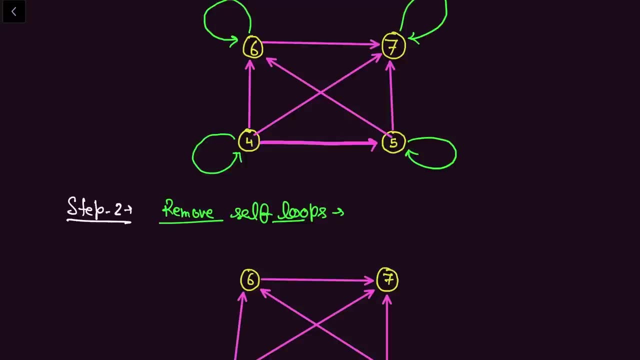 then the second step was that in the second step we will remove all the self loops. so these green self loops, I will mark them and show you. we will delete these four in the second step and we will see the remaining graph. so I have deleted all these green self loops. 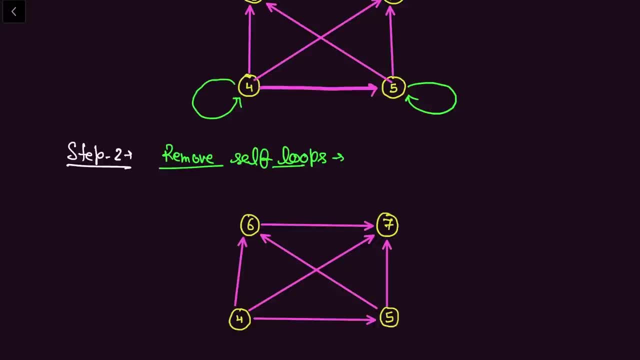 after deleting, we will have this figure in step 2. so we have deleted all the self loops. in the third step: remove self loops. after the self loops, you will have this graph. in the third step we have to eliminate the transitive edges. 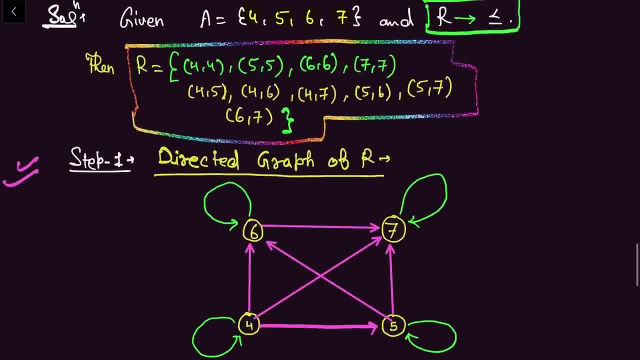 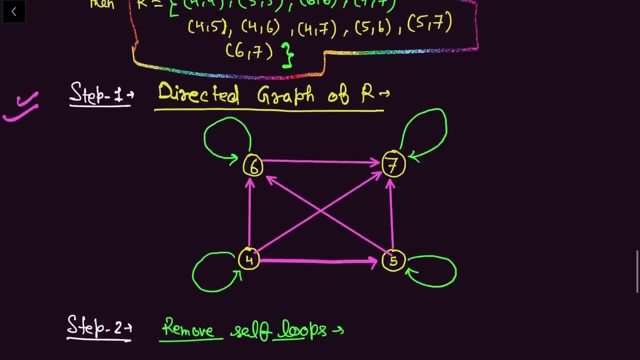 we have to remove them now. see this r relation was 4,4,5,5,6,6,7,7. this is eliminated. let's see the other elements. one is left: 4,5,4,6,4,7. 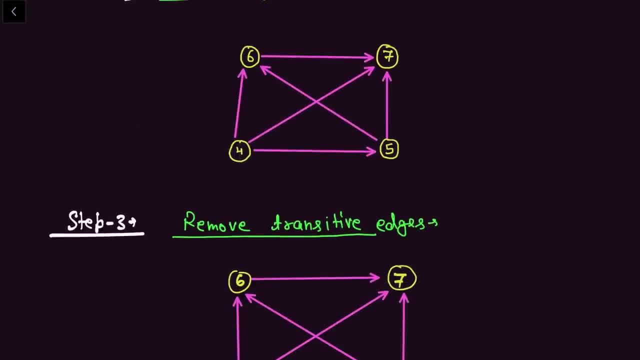 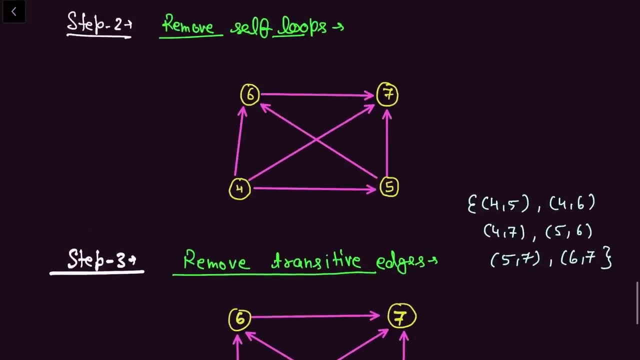 so in relation we have the remaining elements 4,5, 4,6, 4,7, 5,6, 5,7 and in the last, 6,7. I think these six elements will be left when we will delete the reflexive relations. 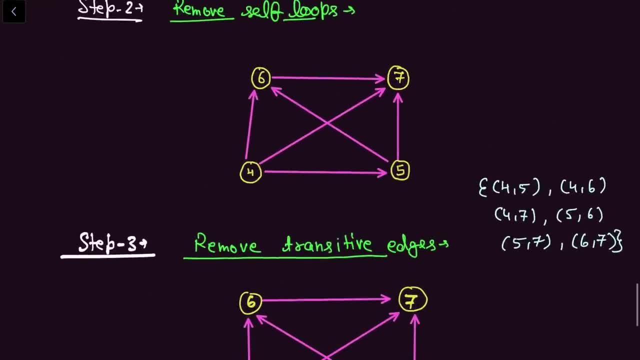 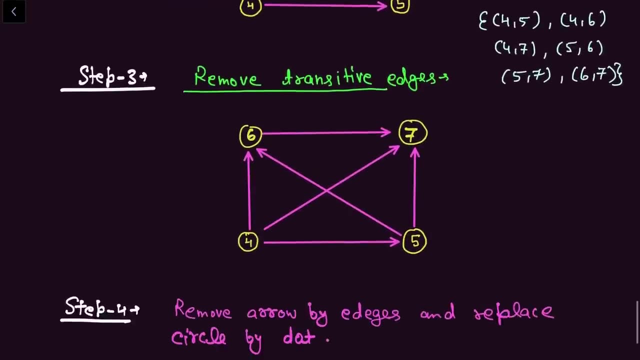 we will delete the reflexive relations 3,3,6,. yes, so in the second step, you have removed the self loops. after removing the self loops in the third step, we have to remove the transitive edges. now, removing the transitive edges is the main work. 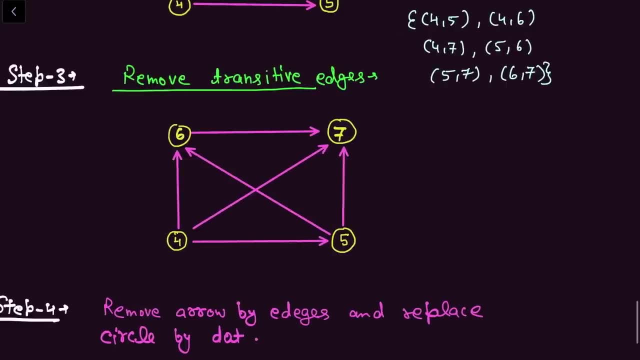 you have to see the transitive relation which pair will be made. if we talk about the transitive relation, then I took the pair 4,5. so 4,5 is related to us, 4,5 is related to us, then the element starting from 5. 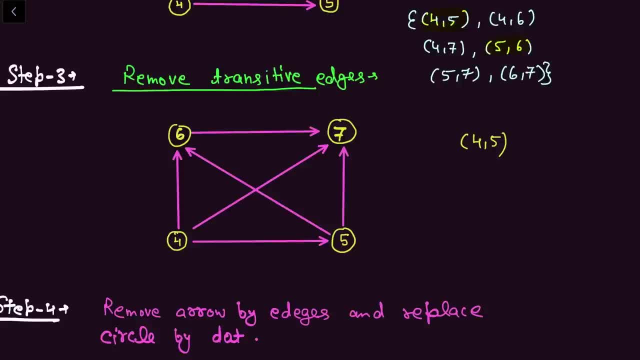 the element starting from 5 is 5,6. right then, I took. 5,6 means 4 is related to 5, 5,6 is related to us. the transitive relation says that the element in the middle will be eliminated, and 4 and 6. 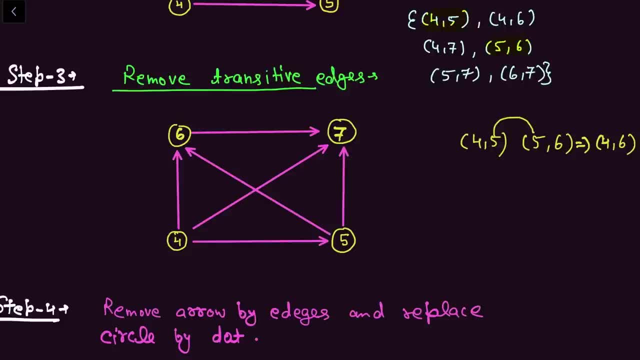 both of them will definitely belong to our set. this 4,6 will definitely belong to our set and this relation- 4,6- is made by our transitive relation and this relation is made by our transitive relation. so the age which we will get from this. 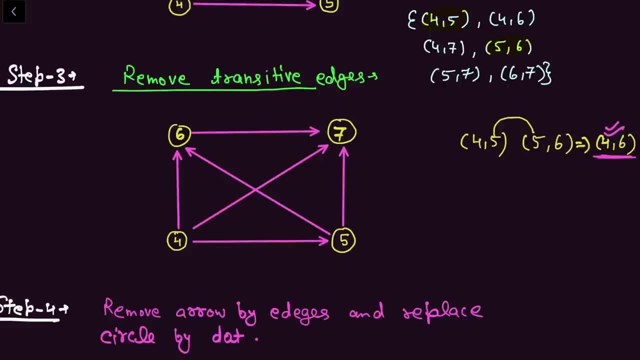 will be the transitive age. we have to eliminate it. so we will eliminate the ages which are made from 4,6. we will delete it. so this is our 4,6. I have deleted 4,6. I will show it again. understand this step carefully. 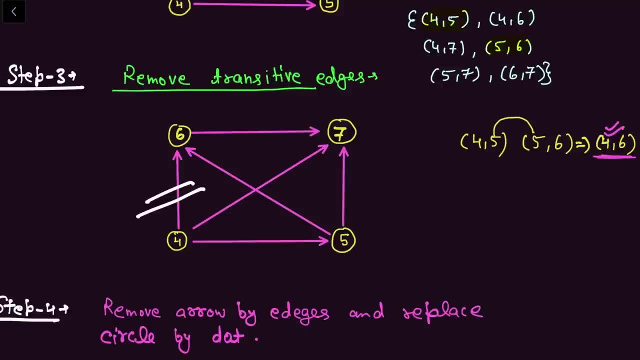 this line of 4,6. this makes the transitive age. in the third step we have to delete the transitive ages. so I will remove this age. see this, I have deleted it. then we have to see which are the transitive relation we will make. 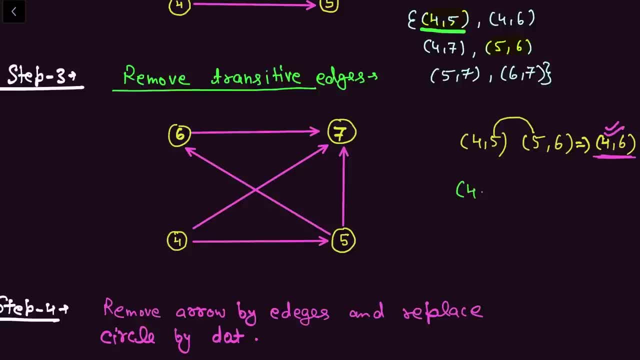 4,5 is in our set. yes, then 5 will start. we have covered 5,6. the other element which will start from 5 will be 5,7. 5,7 is also in our set. this implies now see here also: 4 is related to 5. 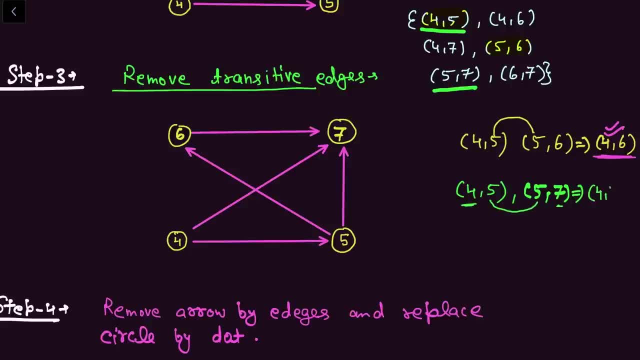 from 5,7. 5 will be eliminated. 4 will relate to 7, so 4,7 will also make transitive age. I will mark the age of 4,7 in the figure. our age of 4,7 will be this: 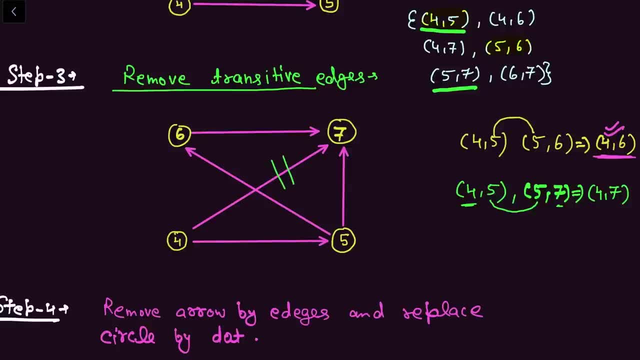 this is our age of 4,7, so this will be the transitive age. I will delete this also. let me delete this also. 4,7 was also transitive age. I have deleted. after this we will see which is our age transitive after this, if we see. 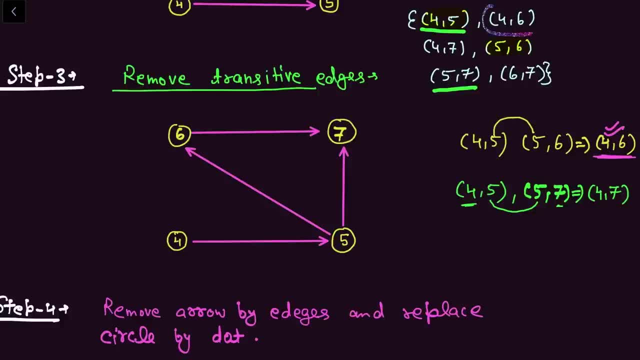 4,7. ok, then we will move to next element 4 and 6 present in our set. then 6 x7 will start. this means 4,6 is also related and 6,7- 6 element will be eliminated. 4,7 means: 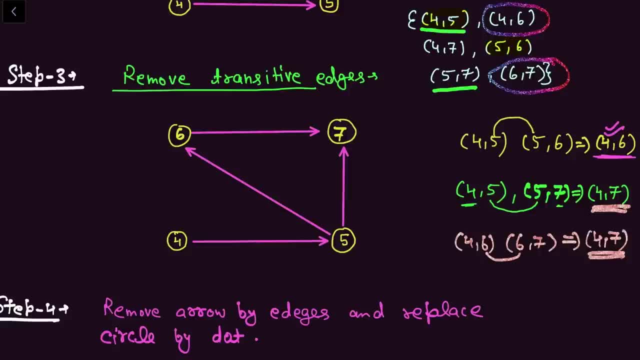 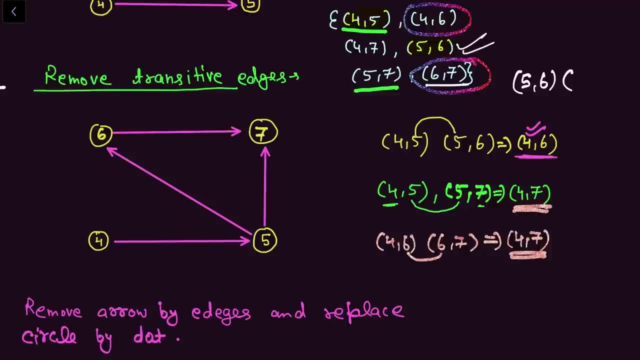 which I have deleted. 4,7 was also here. Let's see which transitive relation can be made. Yes, 5 relates with 6, 5 relates with 6 And 6 relates with 7. 6 relates with 7, So 6 will be eliminated. 5 will relate with 7. 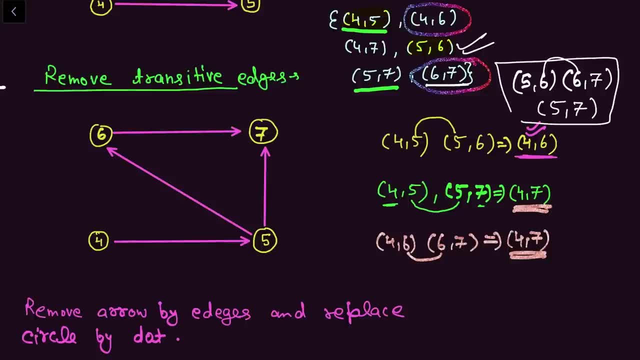 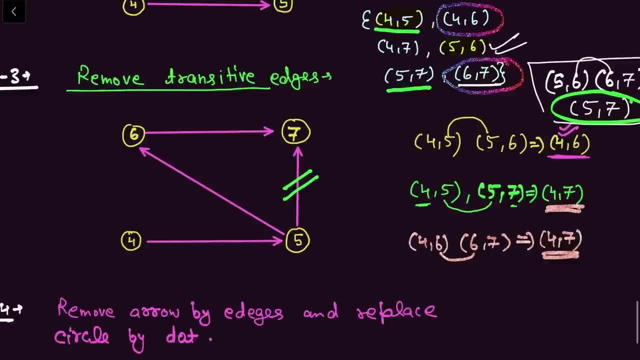 This will also be your transitive relation, So transitive age is going to be made. 5 and 7 are our transitive age. I will show you 5 and 7 in the figure. This is our 5 and 7 age, So we have to remove this too. 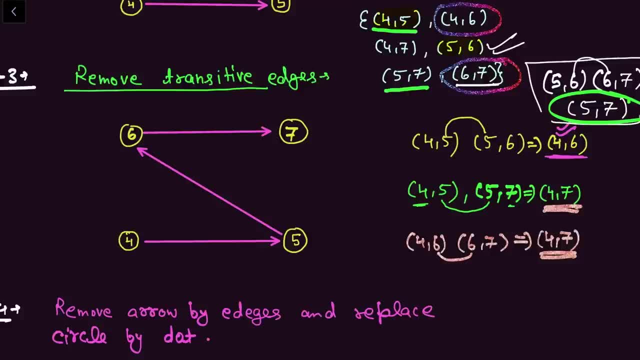 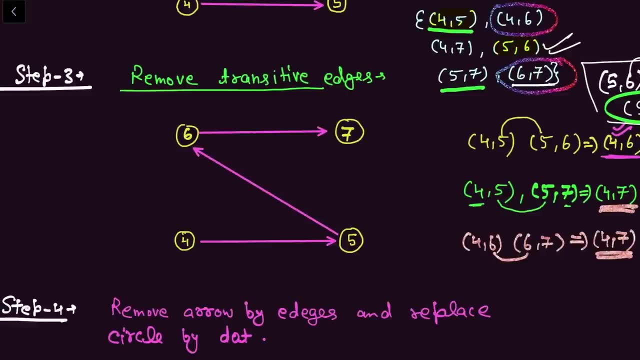 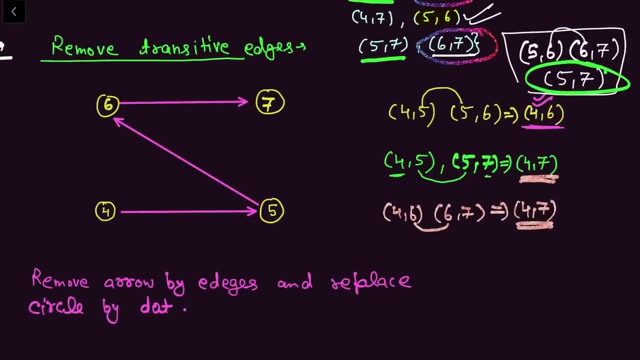 Because this is also our transitive age. So I removed this too. So in the remaining graph you have to see transitive age And eliminate it. delete it. We will not get any other transitive age. We have 3 transitive ages here. I will show you on the side. 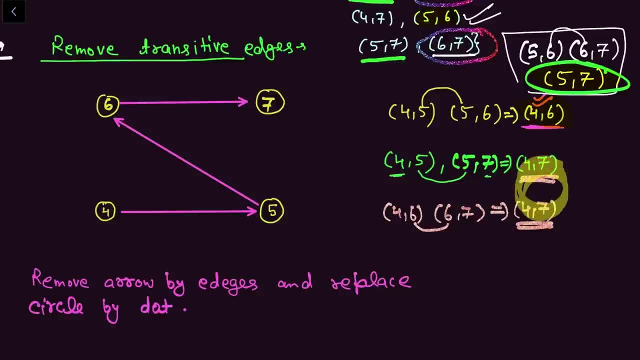 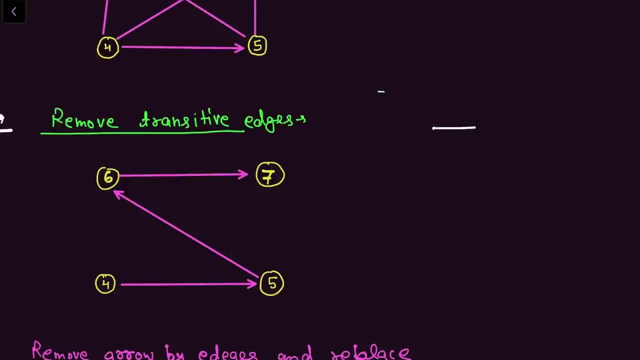 One is 5 and 7, One is 4 and 6 And one is 4 and 7. I deleted all three ages. We will not get any other transitive age, So we have deleted transitive ages. You can write it here. You can tell us the ages that we will delete. 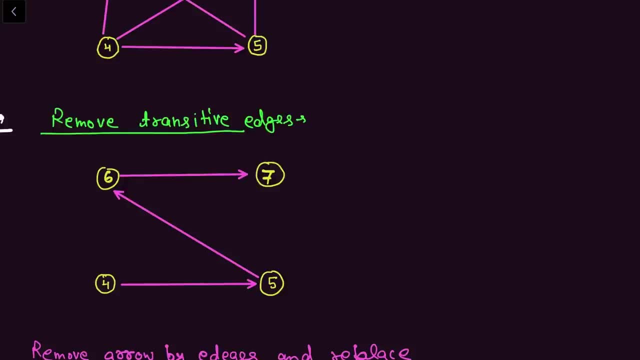 We have deleted. We have deleted 4 and 6. We have deleted 4 and 6. We have deleted 5 and 7. We have deleted 4 and 7. here We have deleted all 3 ages. We have only deleted 3 transitive ages. 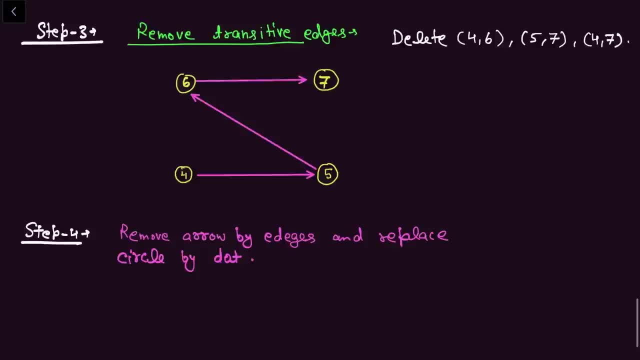 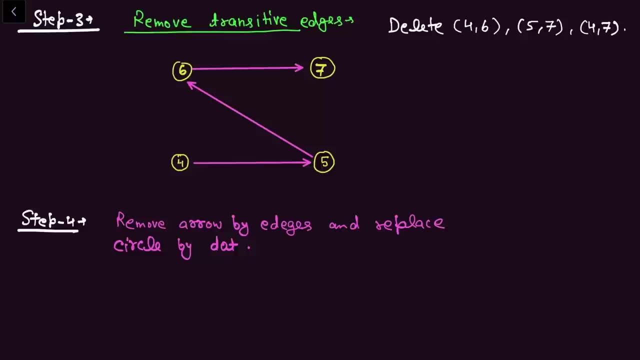 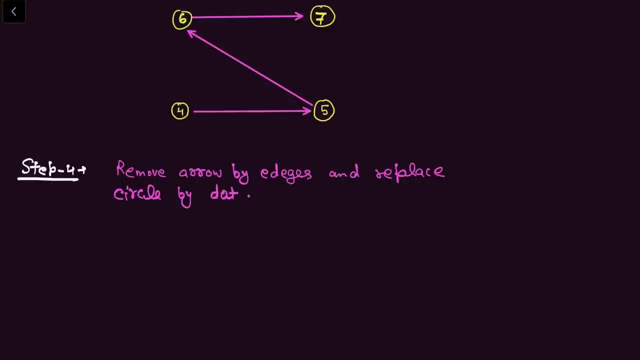 After deleting, this figure will be made in step 3. We have 3 figures used in step 3. Now we are going to draw a doncore line Andfanning Do on arrow. We will use view while trying to obtain. So, according to the arrow, 4 goes to 5, then 5 goes to 6, then 6 goes to 7. 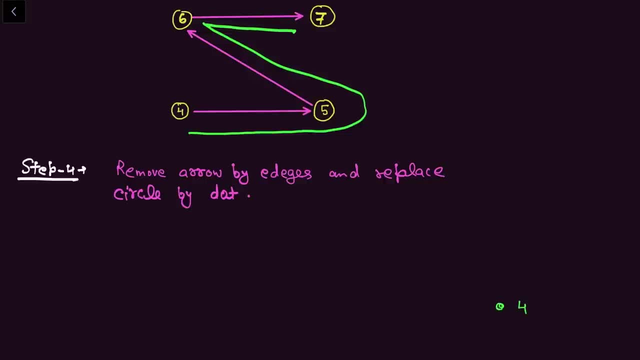 Means we can make a simple figure: 4 goes to 5,, 5 goes to 6 and 6 goes to 7. So this will be a simple figure and we have denoted the circle with a dot. First element will be 4,, this will be 5,, this will be 6,, this will be 7. 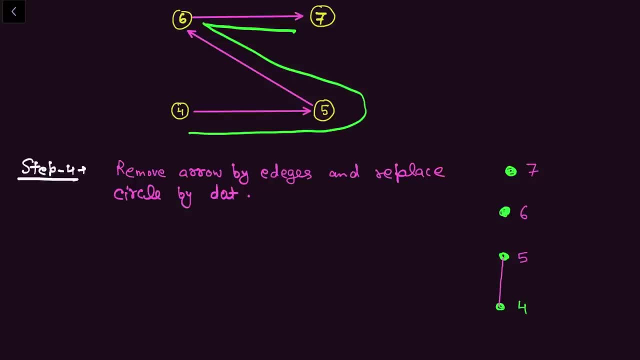 Between 4 and 5, we will take a line above according to the arrow. There is an edge between 5 and 6 and there is an edge between 6 and 7. So this way we will keep it up and keep the lowest element the lowest and the greatest element the highest. 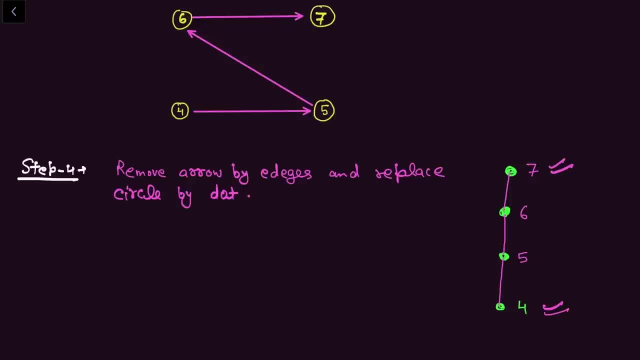 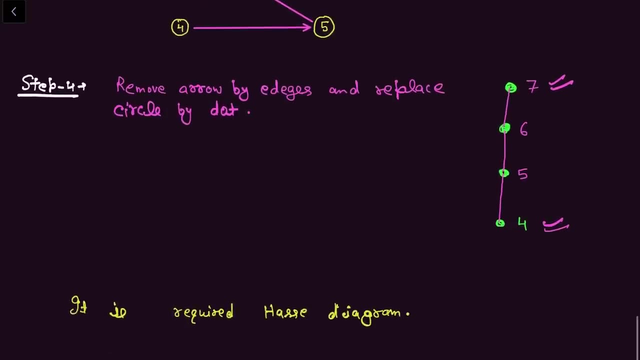 So this is our diagram in the last, in which we have denoted the circle with a dot And, looking at the upward arrow, we changed it to the edges. This will be our required Heisei diagram. Ok, So it does not come to prove that you will make a Heisei diagram or a poset. 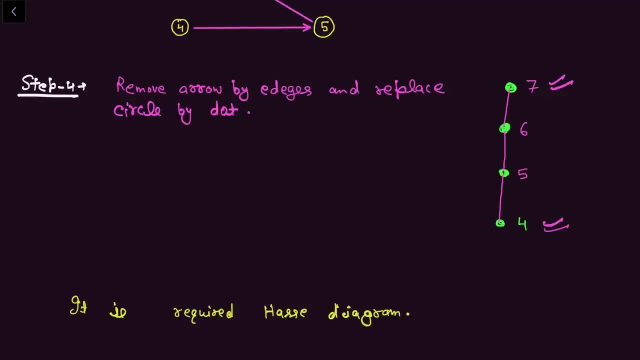 So sometimes it will come in two numbers if it comes. But it has a use. Until you do not know the concept of Heisei diagram, you will not be able to make a lattice. Ok, Looking at the use ahead, I told you the poset. 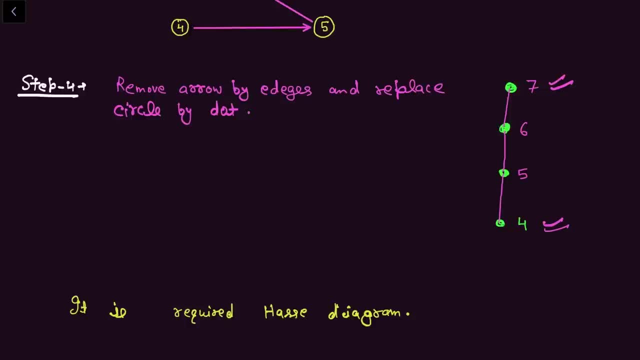 With that we will define the lattice in the next video. Thank you for watching. Students share our channel as much as you can, And you know, in this Engineering Mathematics 1, According to the new syllabus, I have made a playlist. I have to put some videos in it right now. 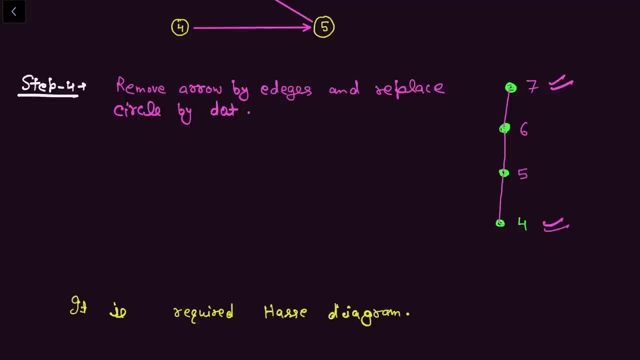 Engineering Mathematics 2,, 3,, 4 And along with district mathematics. your syllabus of discrete structure is available on my YouTube channel. So, students, support as much as you can And tell your friends about our channel.